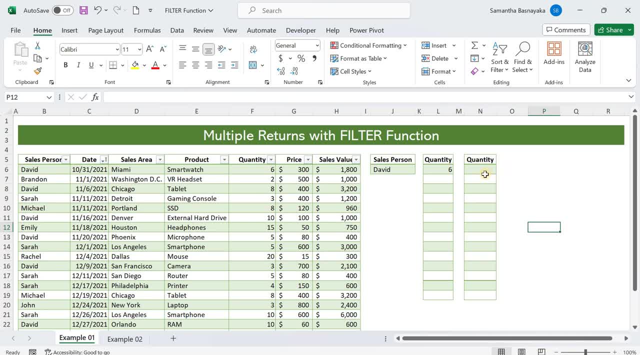 Therefore, in a situation where you want to get all the sales quantities for David separately as an output, it is not possible with the VLOOKUP function. In the early days it was done with the VLOOKUP function by incorporating some other Excel functions like row and match, along with 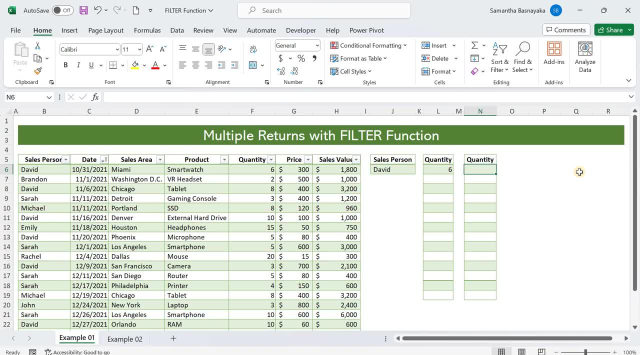 the VLOOKUP function. However, those alternative methods require some substantial effort. As time has passed, Excel has introduced some amazing function that can perform the same requirement with minimal effort. It is another function and the name of the function is the filter function. Basically, 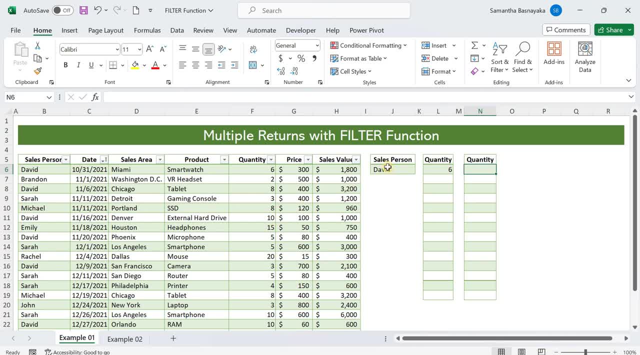 this function is for filtering data from a data table based on criteria, and this function can still be used for our requirement as well. Hence, in this tutorial, we are going to discuss the filter function in Excel as an alternative method to the modified VLOOKUP function, which returns. 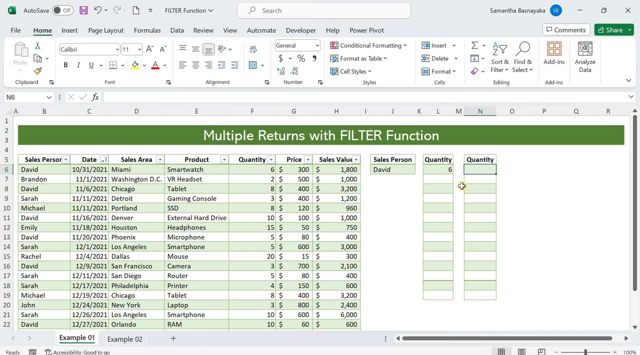 multiple values against a particular lookup value. However, please note that currently this function is only available in Microsoft Office 365 and the online version. Here I will explain to you two examples, and under the first example we are going to look at the filter function. 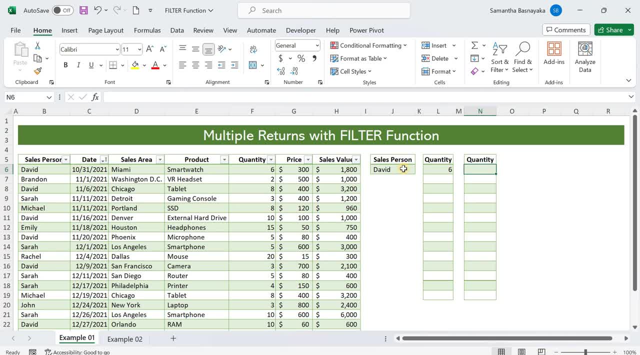 Let's first look at how to get multiple results for a single lookup value. For that purpose, I am going to get all the sales quantities available for David in the sales data table. As the first step, type the equal sign and filter and then press the tab key. Now we need to give. 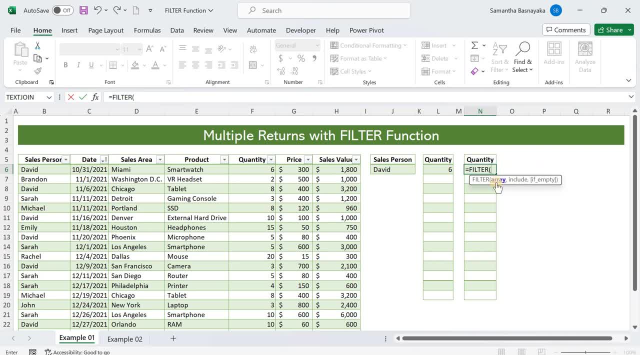 the first syntax criteria for the filter function, and it is array. In this case, arrays refer to the cell range with the values that should come as a result of our function. In other words, it is the sales quantity column. Therefore, select the quantity column from the sales data table and add a comma. 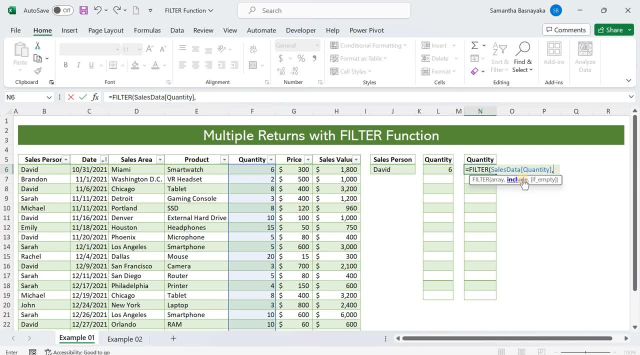 comma, comma, comma. Now, as the second requirement of the filter function, we need to specify the cell range which refers to include. That means it is the kind of criteria that filters the data table. To specify that, select the column that contains our filtering criteria. 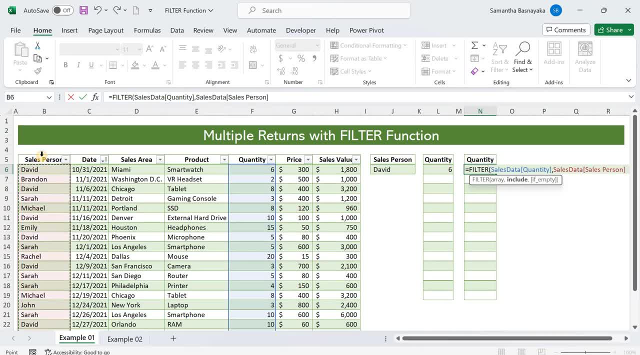 or lookup value. Select the column with the salesperson name and type an equal sign. Then select the cell with filtering criteria or a lookup value and add a comma. Finally, specify what should appear if no output is found for the lookup value. I will add quotation marks. 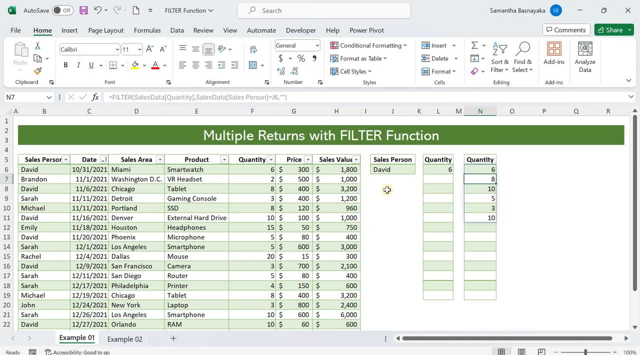 to keep that blank. close the brackets and press enter. Now you can see that all six sales quantities for David are shown as the output. Okay, now we know how this function works, But it would be meaningful if we could get some additional related data, such as date, sales area. 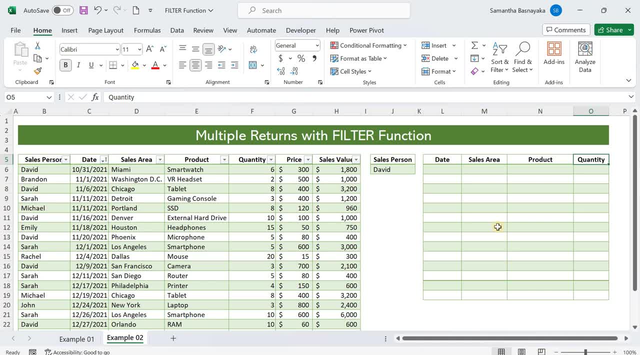 product along with sales quantities. So we are going to look at that in second example and can use the same function for that purpose as well. Just enter the filter function and press the tab key. Here the said related data, such as date, sales area and product, will. 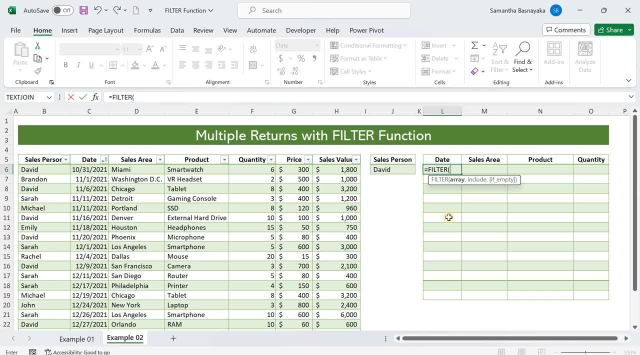 behave as the output or result, like the sales quantities we considered in the previous example. Therefore, those data should come under the array Hence, select all these columns from the sales data table and add a comma. The only difference here is that we are selecting. 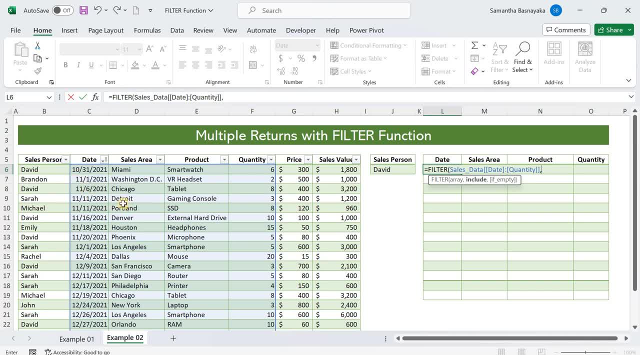 multiple columns as the array instead of one column. Thereafter the steps are the same as in the previous example. Then specify the filtering criteria or the lookup value and the defined output for the blank data, and close the brackets and press enter. Just. 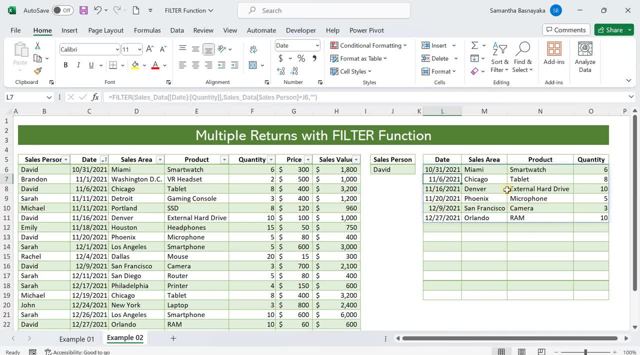 after clicking the enter button you can see all the related data. that also appears in the output for the sales quantities we got for David. Finally, we will check how the output will change if we change the lookup value or the filtering criteria For that. 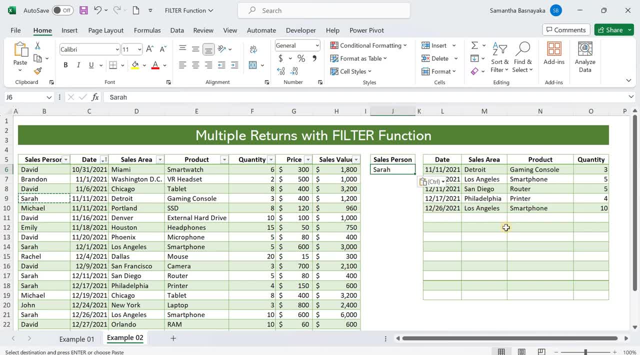 I will copy and paste the salesperson name, Sarah, in cell J3.. You see, now the output has changed and you have successfully retrieved multiple values for a single lookup value with the help of the filter function. This is what I just wanted to share with this tutorial.